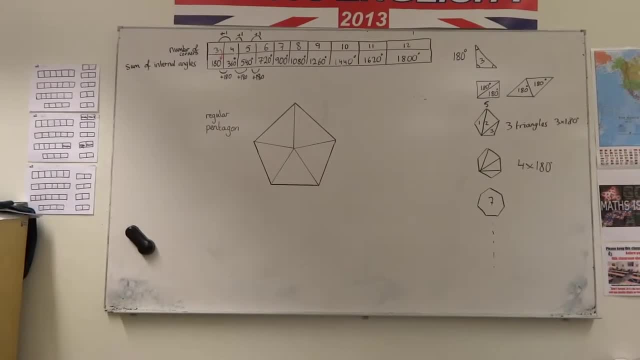 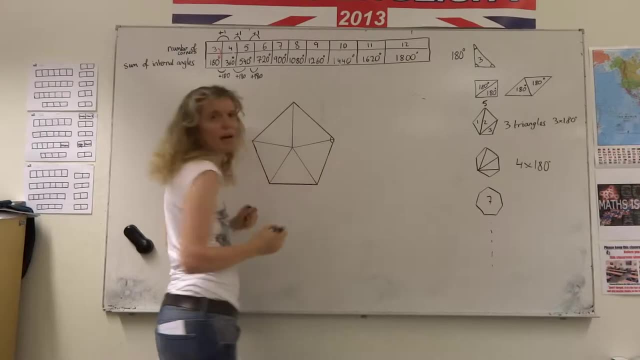 Okay, the question here is to find out the angle. Was it this angle you had to find out? Yeah, So you need to find out this angle. And how would you do that for a pentagon? Well, this again is where your skills and understanding of triangles come in. 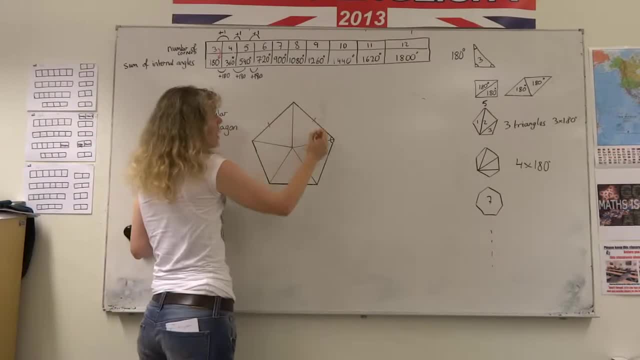 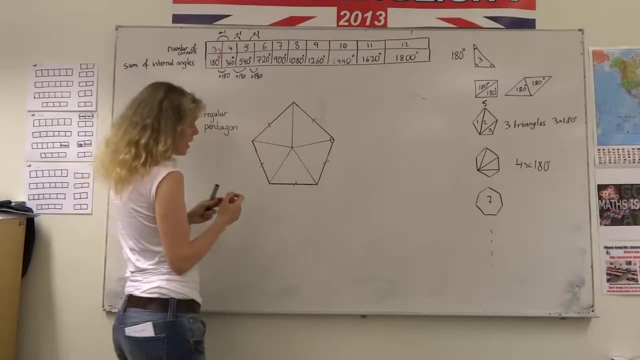 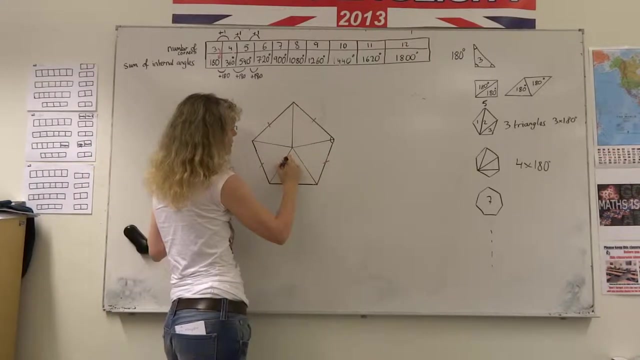 This is a regular pentagon. It means that all of these sides here are the same length. This is going to build us a triangle where, if this is the same length on all of them, the lengths of these angles here, these lines here- sorry- they're also going to be. 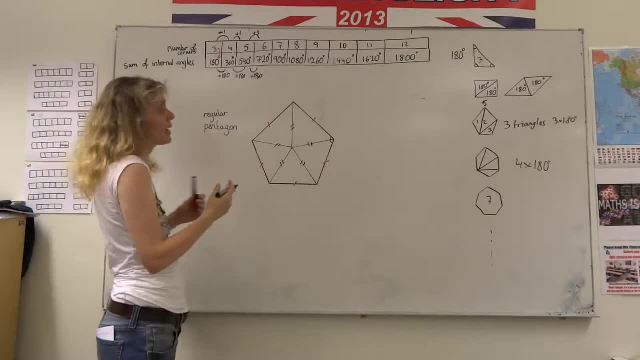 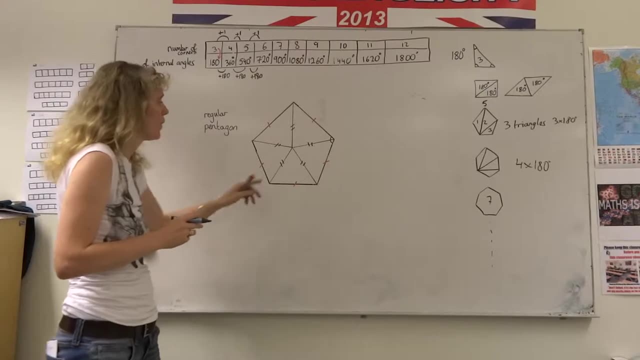 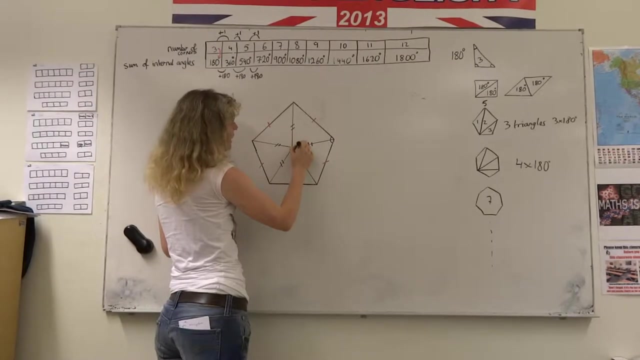 the same length. So when it's a regular pentagon, we are going to get like an isosceles triangle here, where these lines here are the same length. So when it's a regular pentagon, lengths are going to be the same. so the first thing we need to think about, okay, is: we know that. 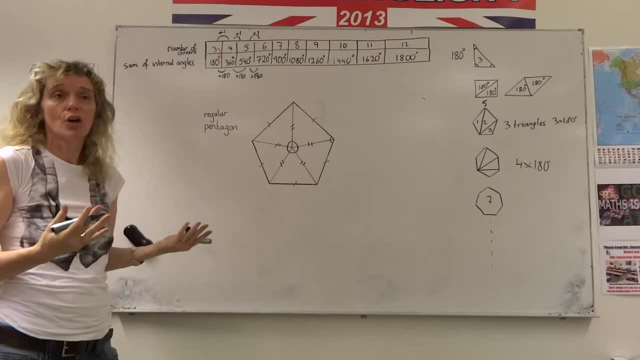 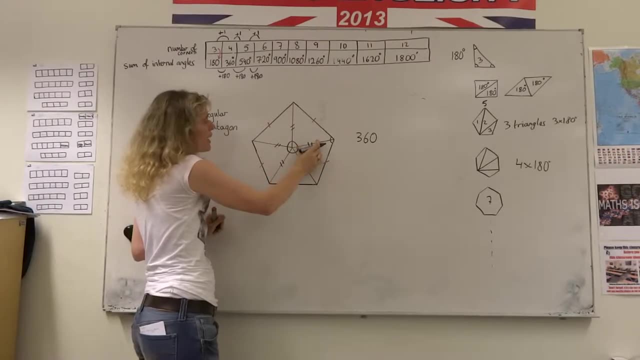 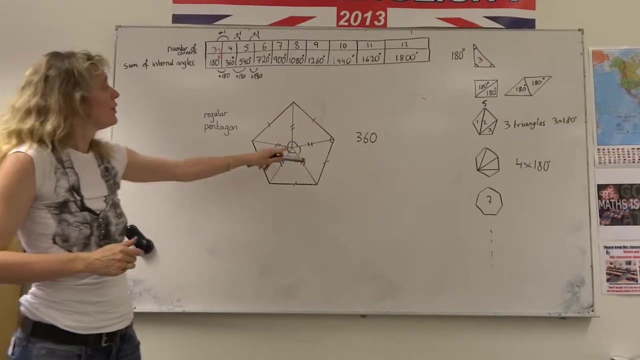 in if we were to measure the angle of the whole of this. it's a circle, internal angle it's going to be 360 degrees, but we split it up into five different triangles. so if we would like to know this particular angle, just this one here, what is the angle? and they're going to work out to be 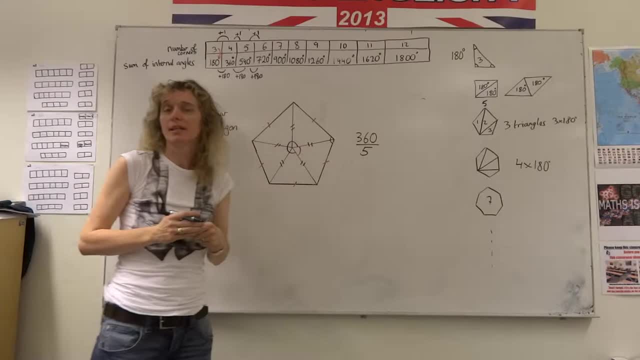 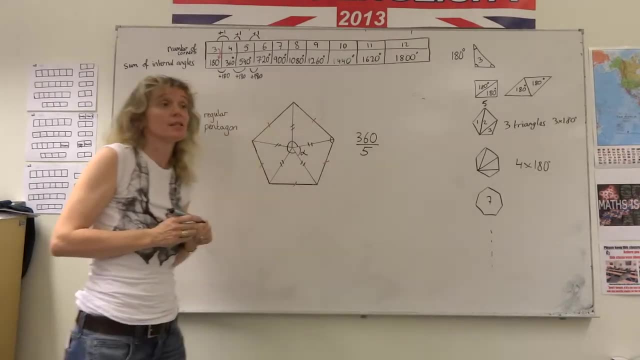 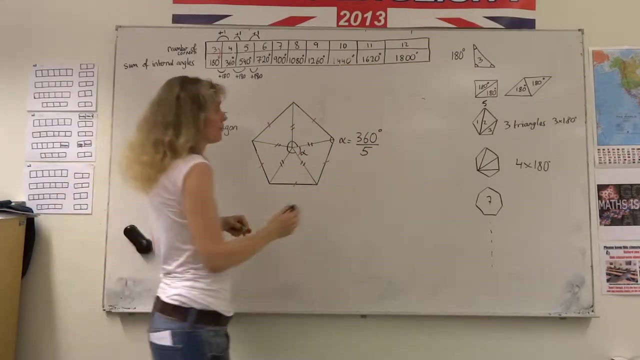 well, it's going to be a fifth of 360. so this little angle here, the red one, let's call it angle alpha. we often use greek letters for angles. the angle alpha is going to be 360 degrees split up into five. well, five goes into 36, seven times, with one left over. five, seven to 35, and we have 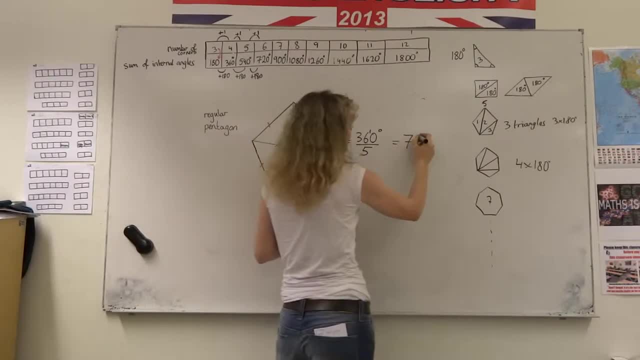 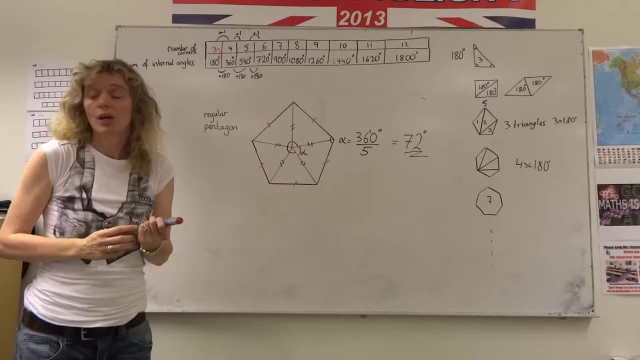 36, so there's one left over and five goes into 10 two times. so we get an angle of a alpha to be 72 degrees. now we have to look at the rest of our triangle, because what do we know about the rest of our triangle? 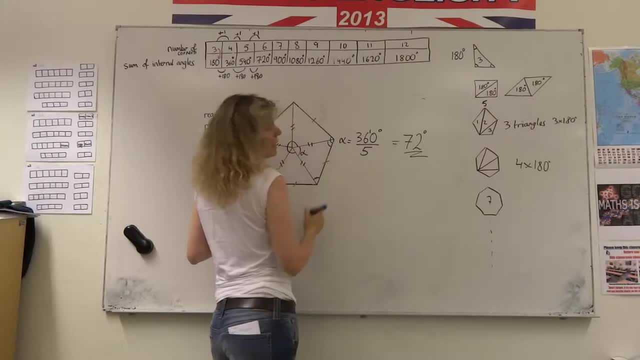 well, we know that this angle here, plus this angle here in our triangle, must be identical, and each of these must be 180 minus 72 divided by 2. so our angle, let's call this angle beta. our angle beta is going to be the angles of the triangle.